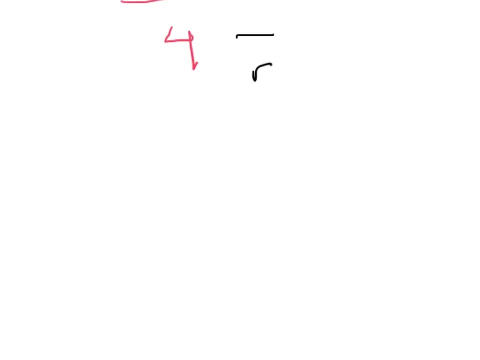 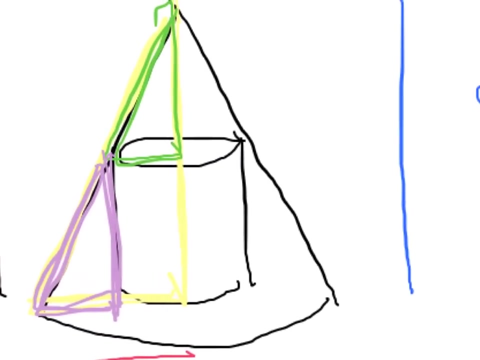 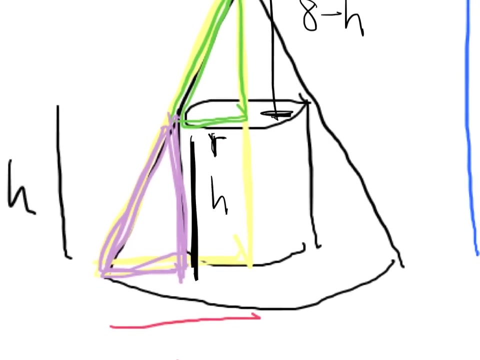 Okay, what can we do with that observation? Well, let me zoom in accurately here: This is r And this distance is 8 minus h. Likewise, this is h And this distance is 4 minus r. Now the question is: 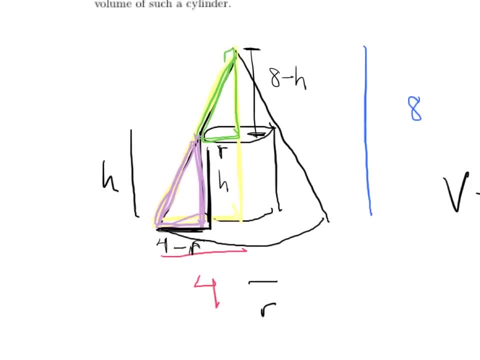 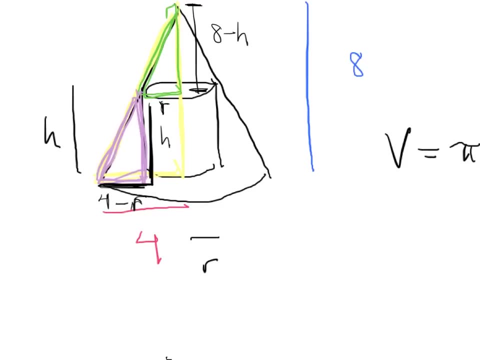 what do we know about the big triangle? The easiest way to phrase what we know is in terms of slope. The slope of this line is: the slope of this line is 8 over 4.. So the easiest thing to use actually, then, is going to be: 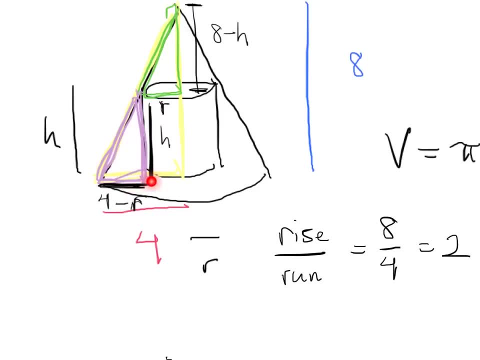 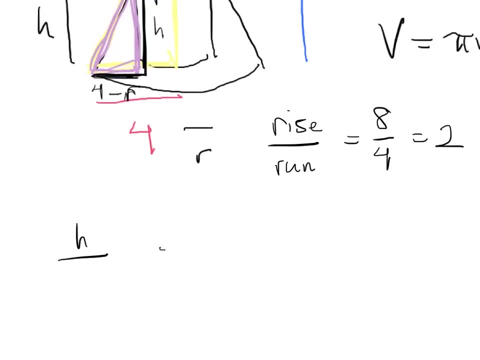 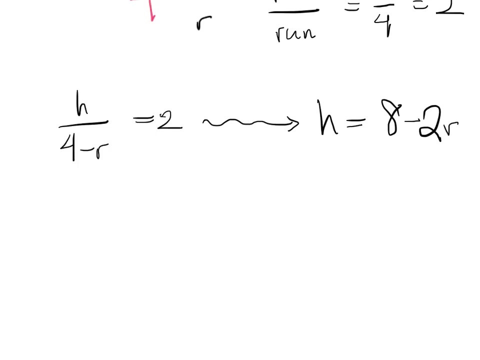 h over 4 minus r equals 2.. And that tells us that h equals 8 minus 2r, And that's all we need to get volume in terms of one single variable. Okay, so I'm going to finish this out here. 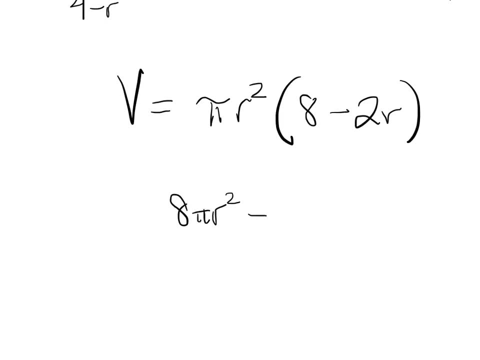 8 pi r squared minus 2 pi r cubed. Let's take the derivative: Okay, 16 pi r minus 6 pi r squared, That's the same as 2 pi r times 8 minus 3r. If we're setting that, equal to 0,.